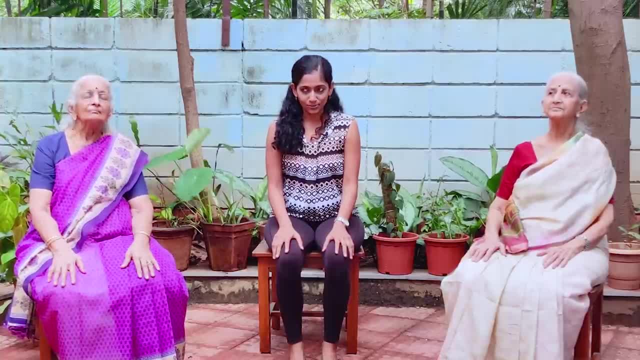 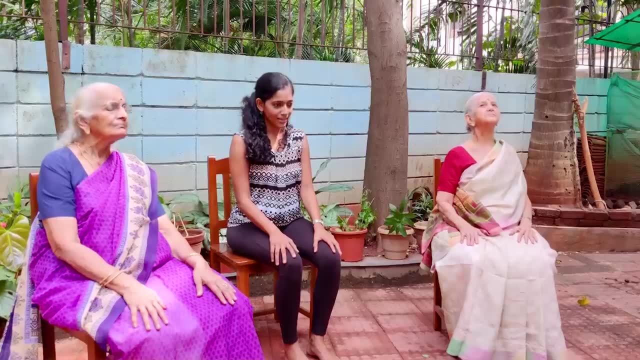 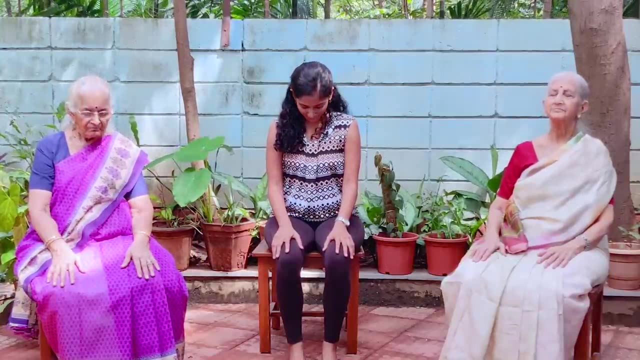 up, Exhale down. Inhale up, Exhale down. Inhale up, Exhale down. Inhale up, Exhale down. Now slowly look straight and tilt your head to your right side. So tilt, so that your ear is close to your shoulder. Come back centre. Tilt to your left. Tilt to your right. Tilt to your left. Tilt to your right. Tilt to your left. Tilt to your right. Tilt to your. 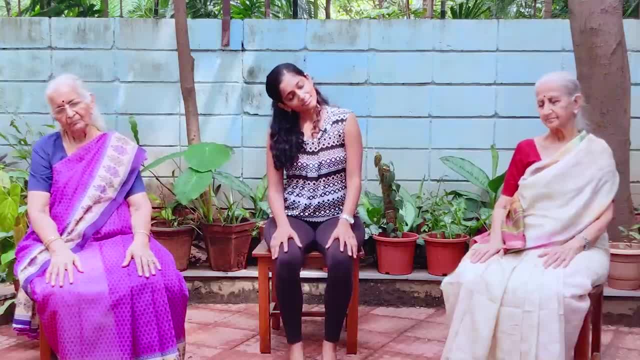 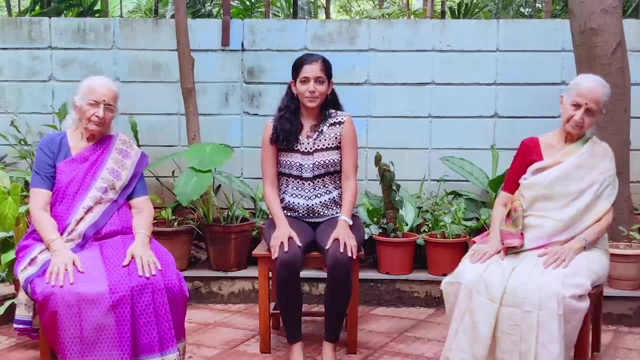 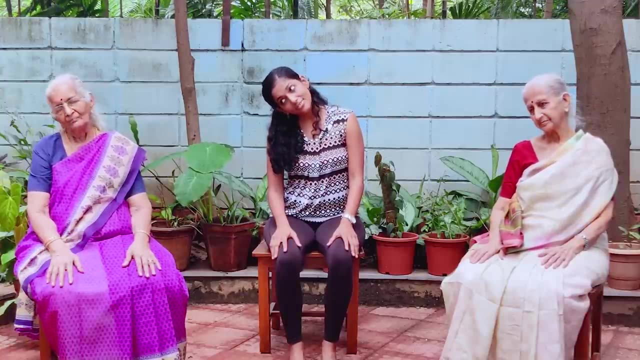 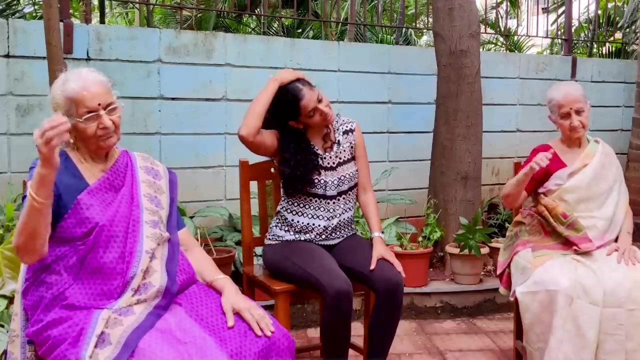 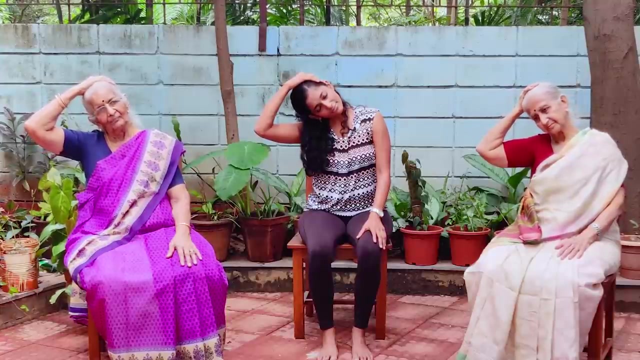 left. Slowly. come back centre. Now once again, tilt to your right side and stay on your right side. You can keep your right hand on your head and pull your head closer towards your shoulder. Come back to the centre. Do the same thing on the left. So tilt to your left and keep. 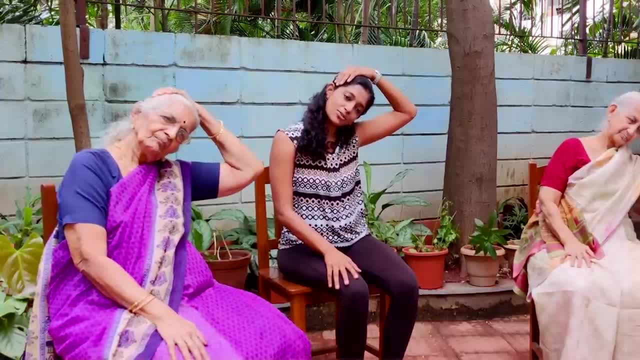 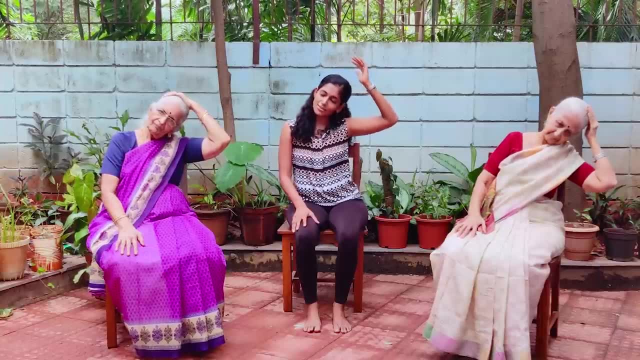 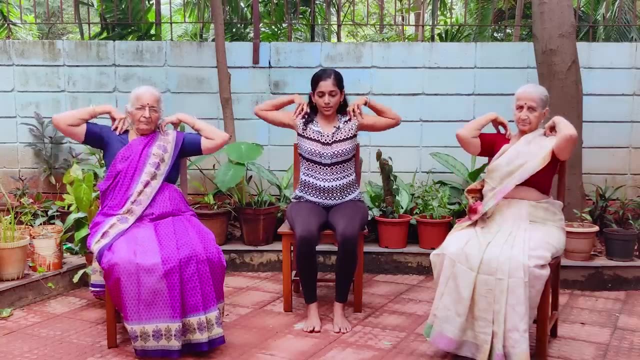 your left hand on your head and pull your head closer towards your shoulder And slowly come back centre. You can keep your hands on your shoulders. We are going to start rotating your elbows going around, So first going to the back, Keep breathing normally. 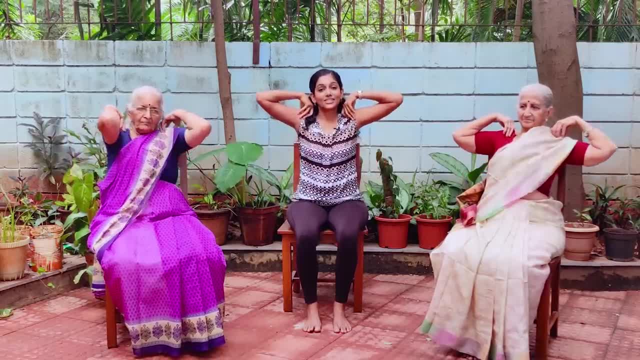 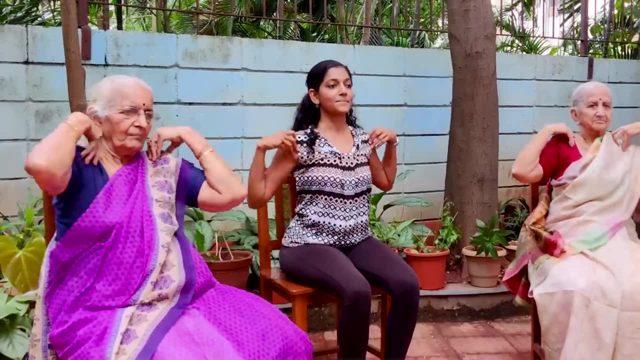 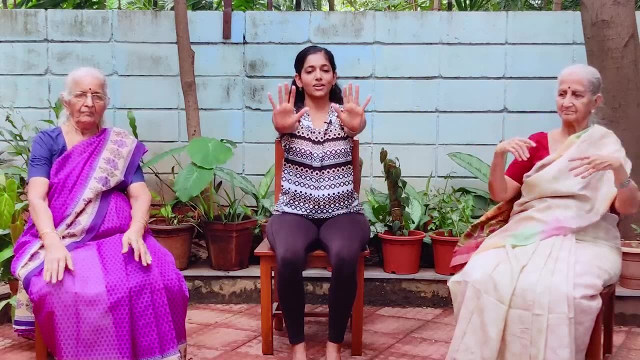 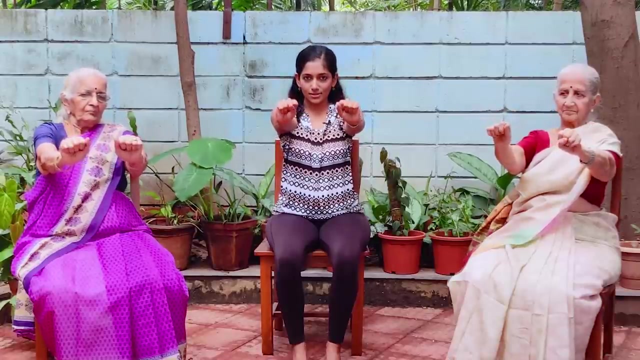 And we will slowly reverse, Going the other way, And relax. You can stretch your hands in front of you, open your fingers wide and we will close and open, and close and open and close, Open, close and open. And now we will do the same thing on the other side. We will start with the right side And 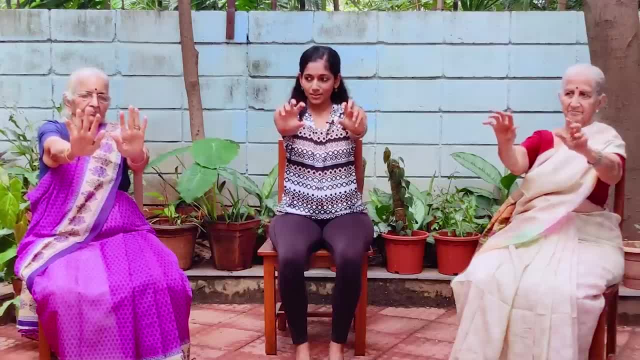 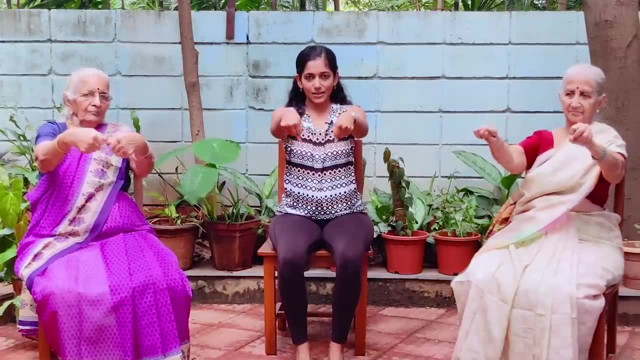 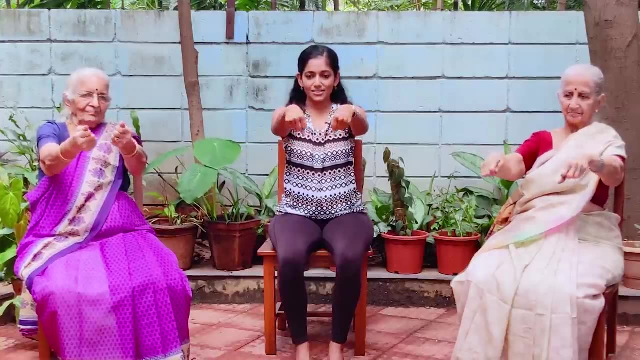 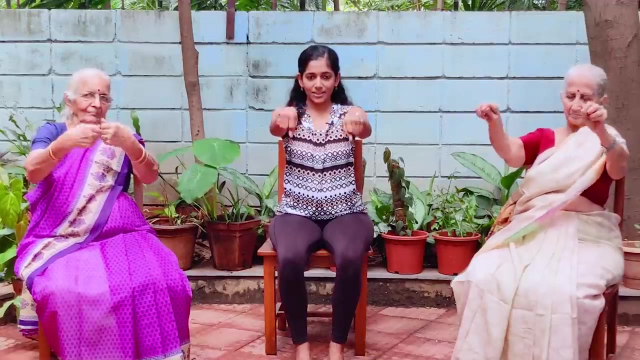 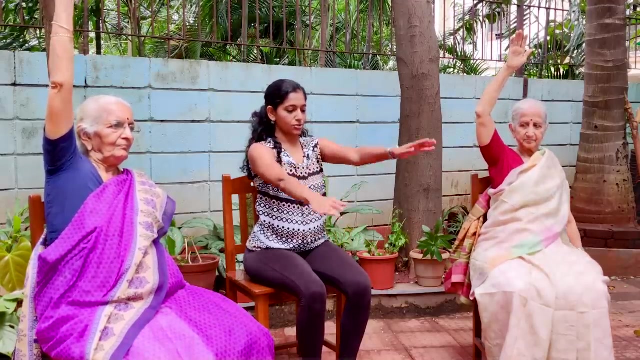 close open, close open and stay closed and let's rotate your wrist making circles and reverse other way. very nice, slowly get your hands down. now raise your right hand up and keep your left hand down, right hand up, left hand down and switch left hand. 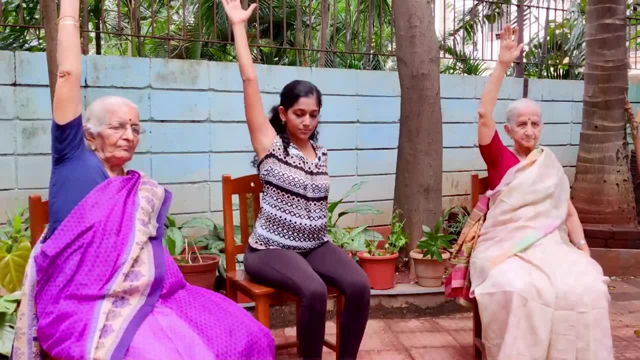 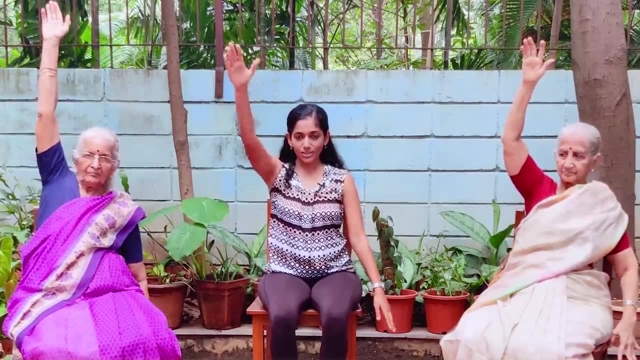 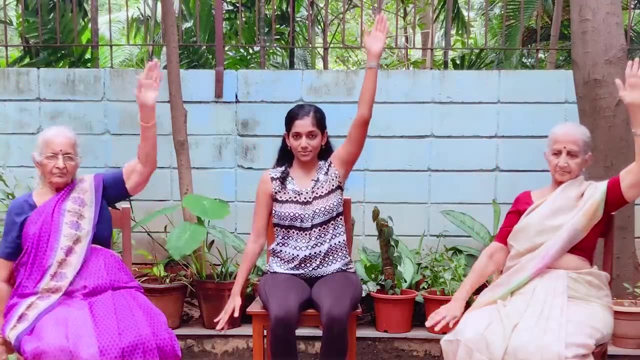 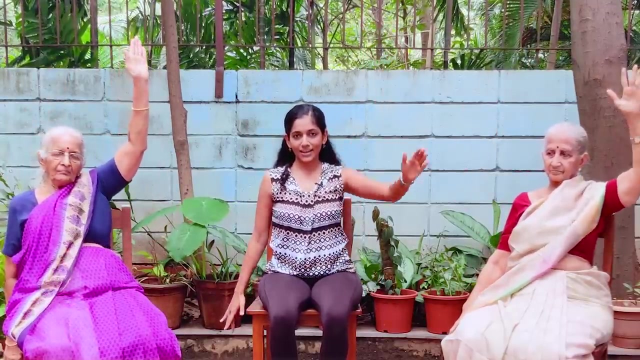 up, right hand down and switch and switch, switch, switch, switch and switch. two more times: right hand up, last time, left hand up and relax. Now, from here you're going to stretch both your hands out to the sides. 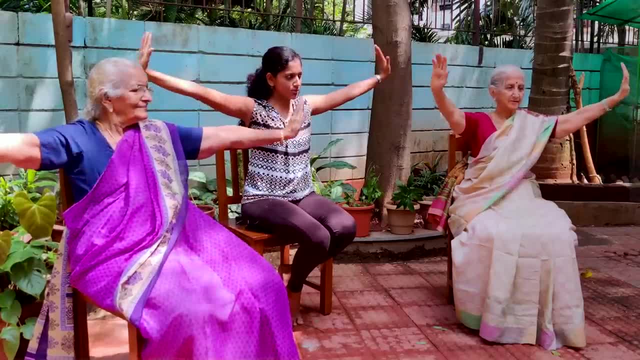 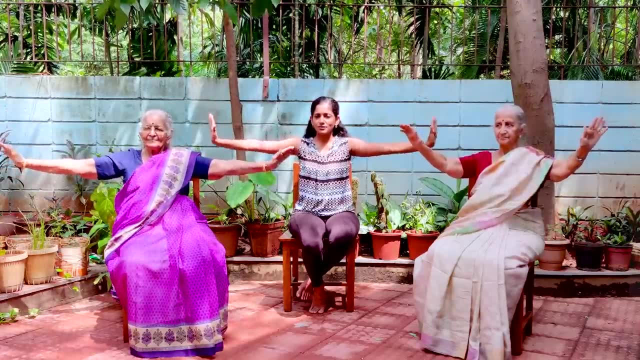 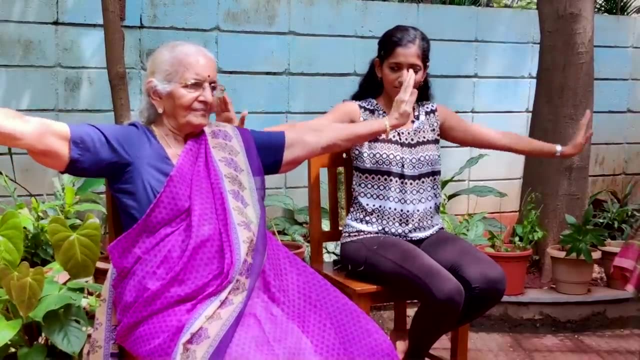 keep your fingers pointing up and we'll make small circles going: 1,, 2,, 3,, 4, 5. reverse 5, 4, 3, 2, 1. reverse again: 1,, 2,, 3,, 4, 5. last time, reverse 5,. 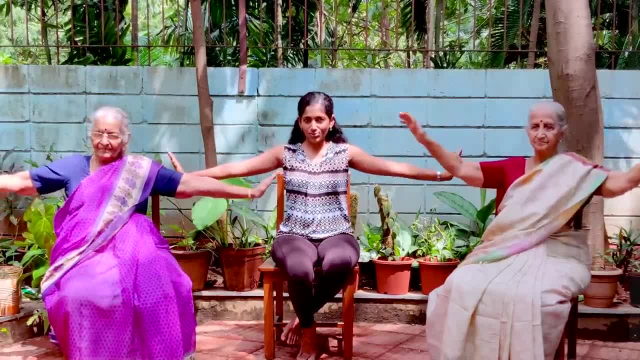 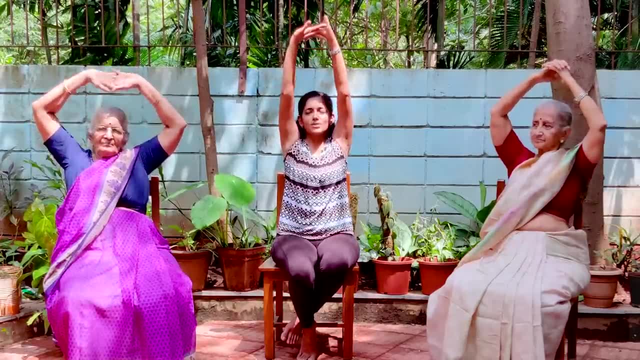 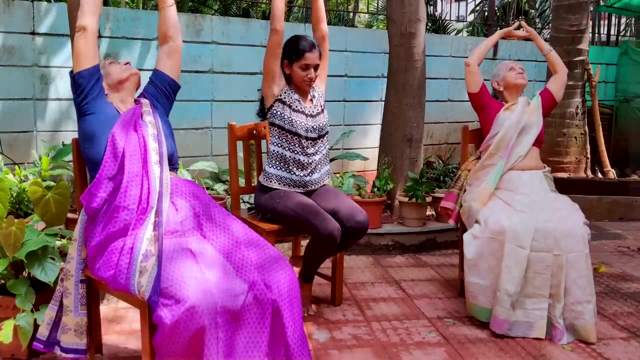 4,, 3,, 2,, 1 and get your hands down. now once again, raise your hands up, hold your fingers at the top, let your palms face up and stretch, stretch, stretch. keep your back straight, keep stretching. now look up with your head and look down once. 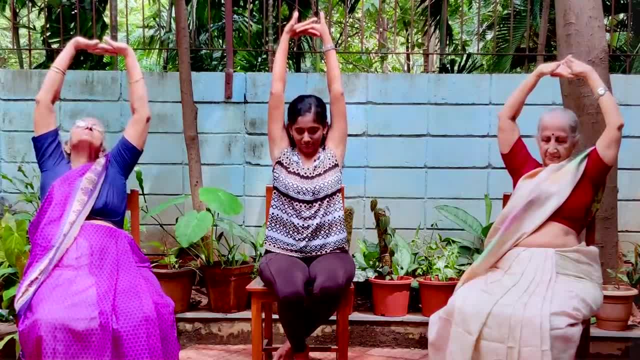 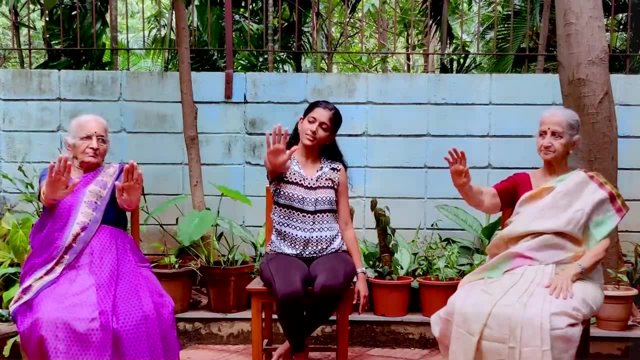 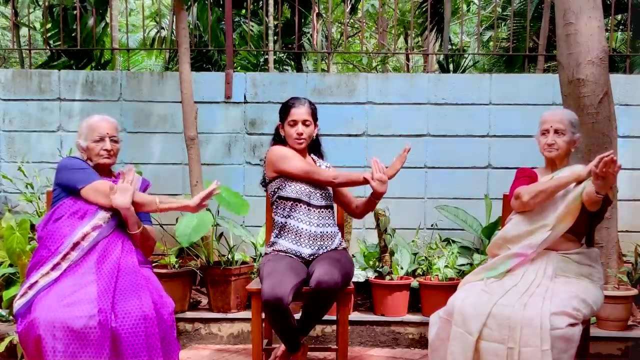 again. look up and look down, slowly, get your hands down. you're going to stretch your right hand in the front, only your right hand, okay, And take your right hand to the side. keep your left hand in front of your right and pull your hand. keep your left. 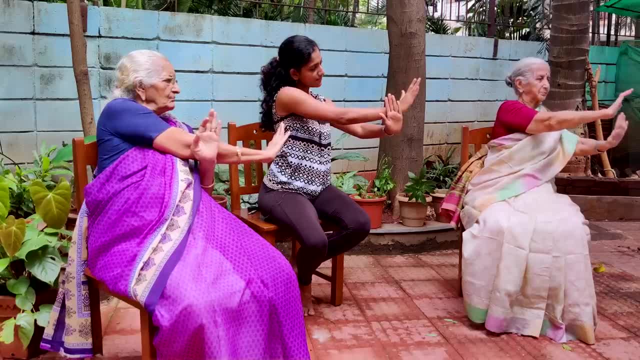 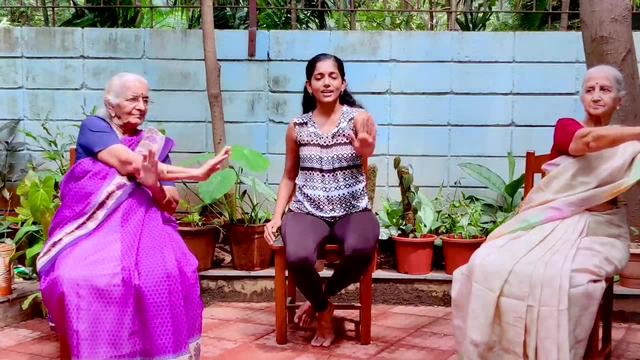 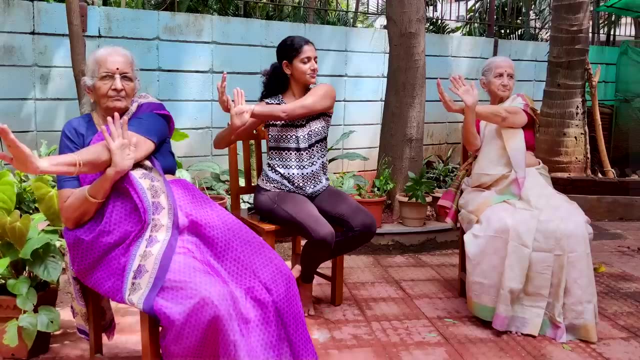 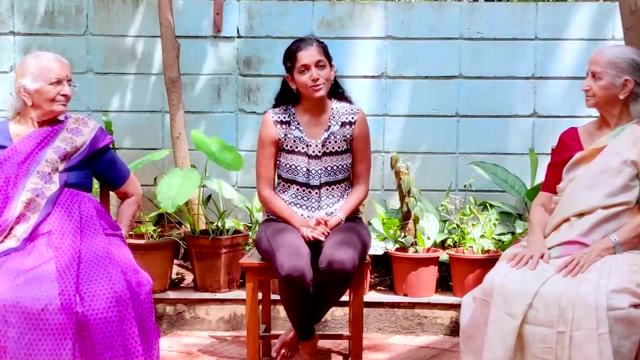 hand in front like this and pull on the other side- left hand up, right hand on the outside- and pull slowly, come back and relax. the next thing we're going to do is few twists and stretches for your spine. okay, we're going to stretch to the side now, so you're just 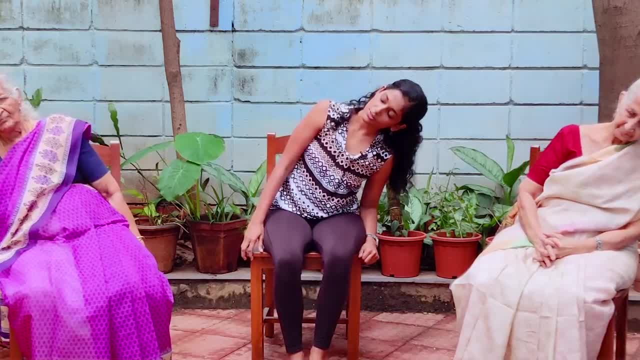 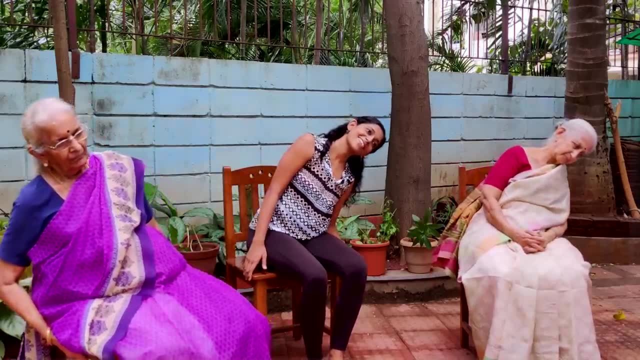 going to go from side to side. you hold the chair if you want to and you can slowly go to your right and to your left. so as you exhale, you go to the side inhale, you come Center, exhale to the side, inhale to the center, keep going. 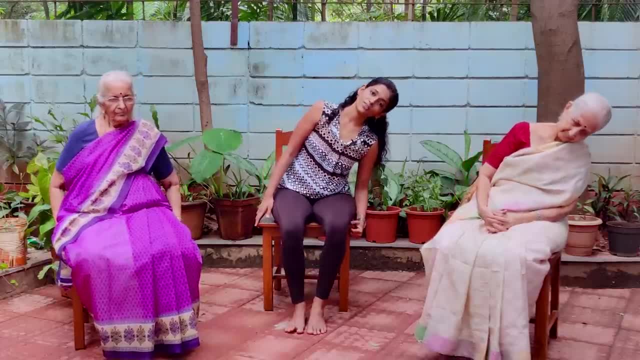 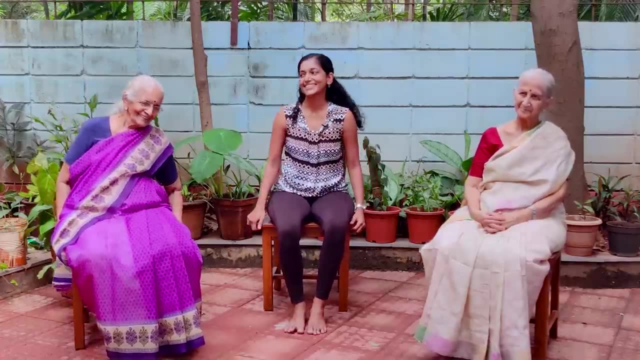 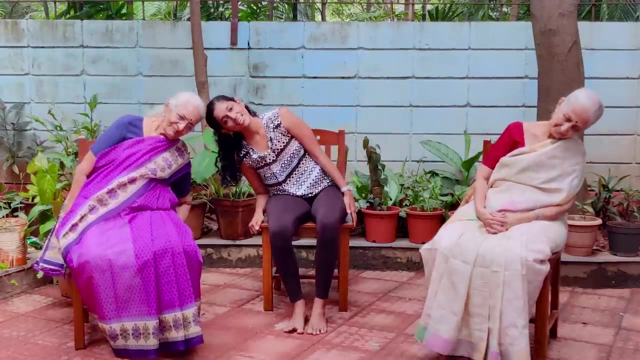 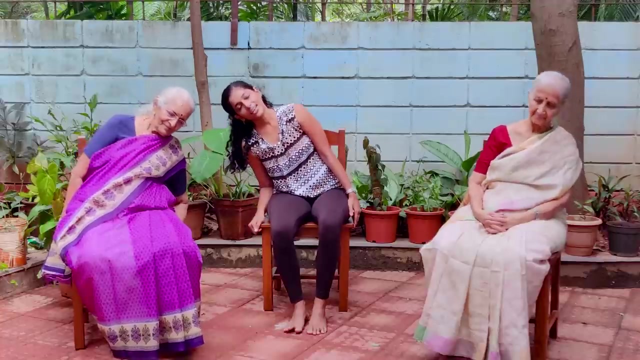 going one side at a time. keep going from side to side with a gentle smile on your face. keep going. so exhale to the side, inhale Center. exhale to the side, inhale Center. exhale to the side. last two times, to the side and Center, last time with 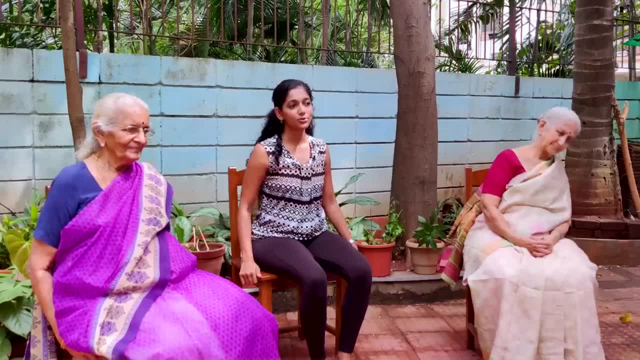 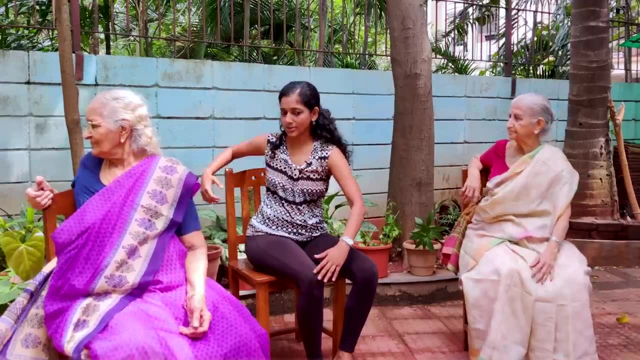 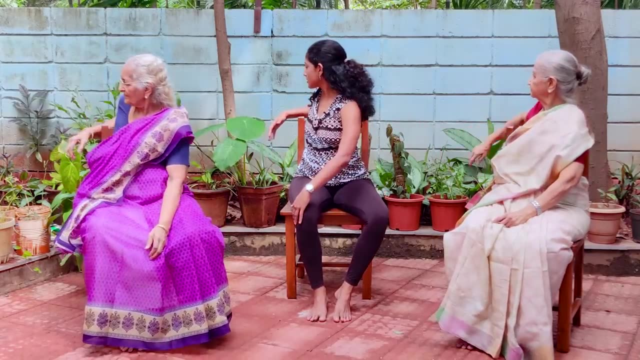 the side and come back Center. now, from here we're going to twist and look behind. so you hold the chair behind you, slowly twist and look behind and come back to the center. do the same thing on the other side: twist and look behind, come back Center again. twist, look behind you, come Center, twist, look behind. 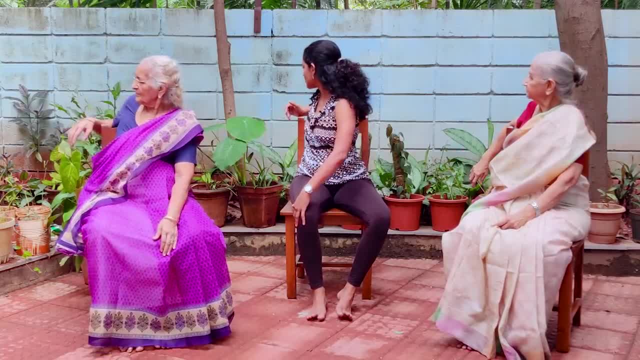 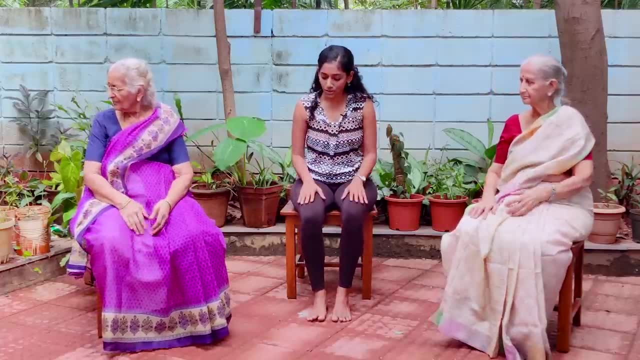 you come Center two more times. twist the back, come Center one last time. twist and come Center. okay, we're going to work on our legs now. so you raise your right leg up only one leg at a time. so we'll just point and flex your toes. so 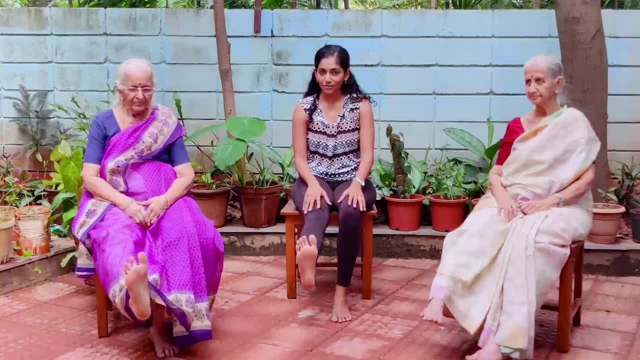 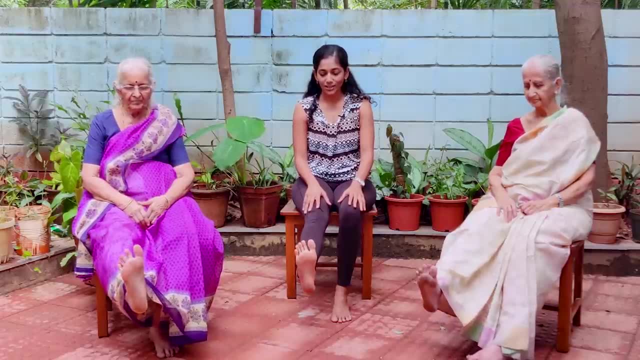 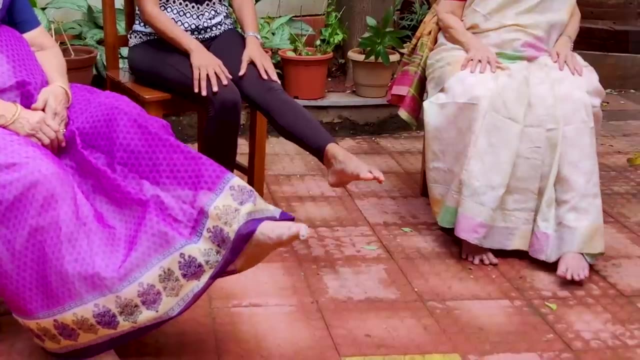 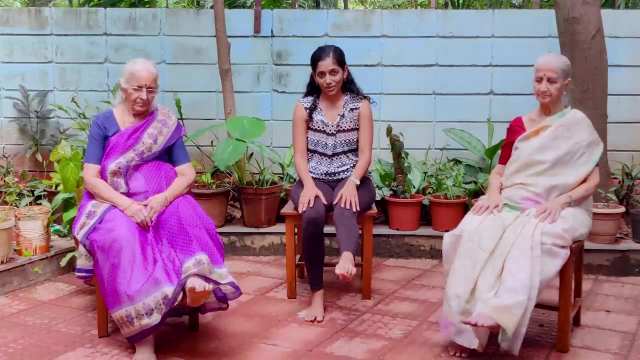 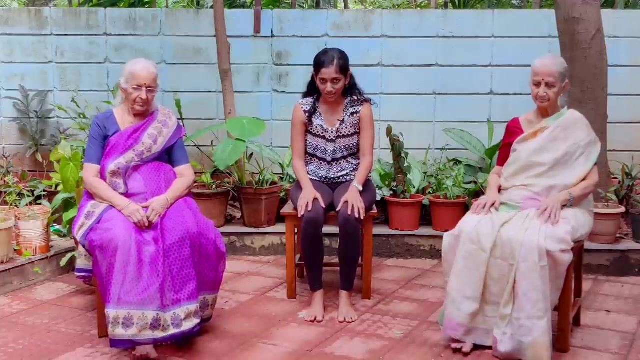 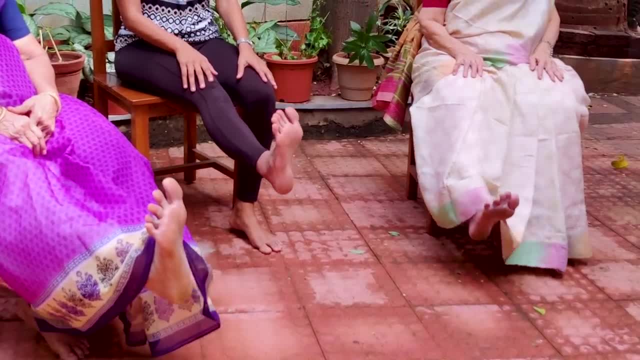 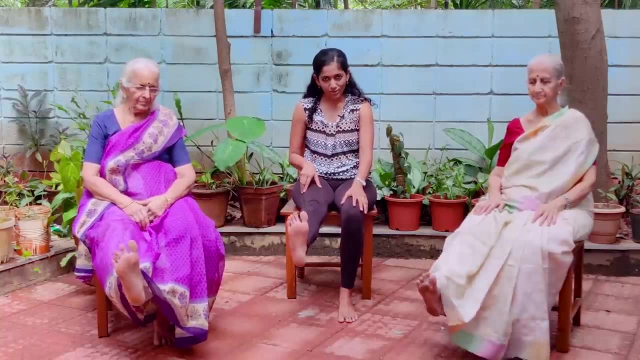 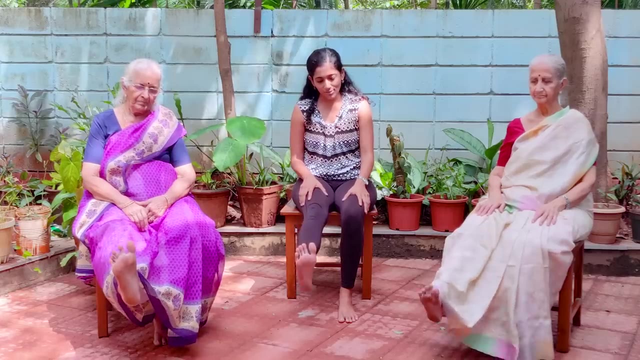 and you flex your foot and we'll just start kicking up slowly. so sometimes, when we are older, our knees tend to give up on us. so we are doing these exercises to strengthen your thighs, so that your knees will also get strong. we'll just keep pushing it up and slowly come down, relax with on the other leg. 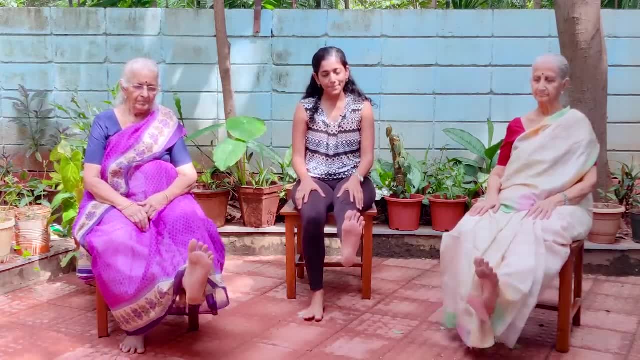 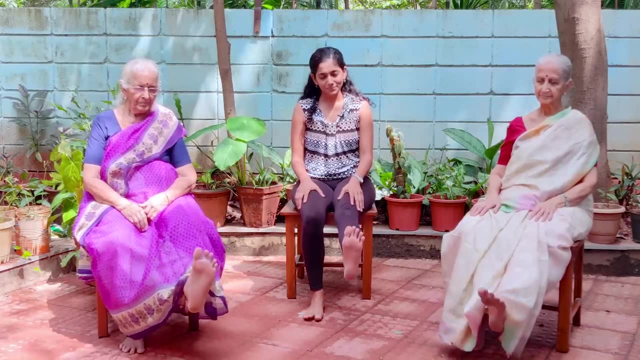 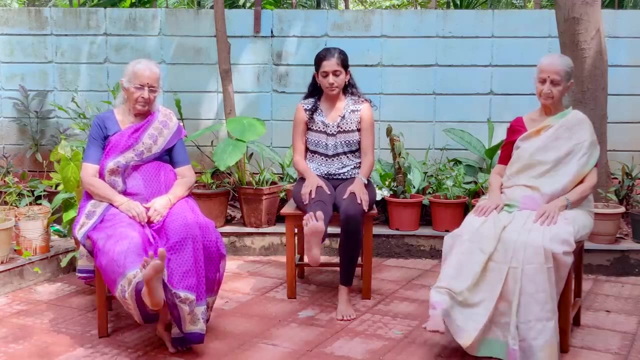 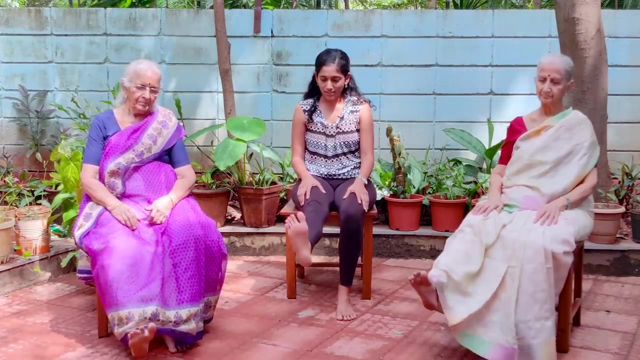 flex your foot and push up. so you keep your foot flexed and you keep pushing it up and relax. okay, again, right leg, flex your foot. you'll make small circles. you want to try and keep your knee as straight as possible and reverse on the other side. 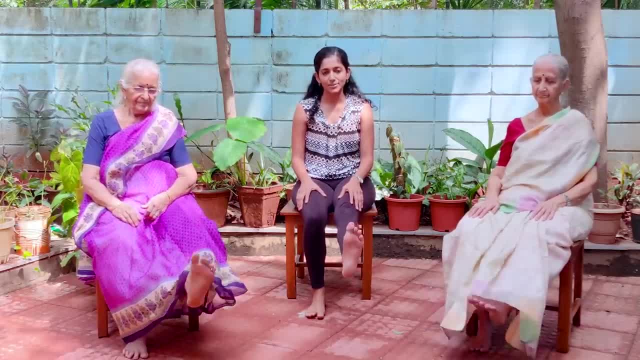 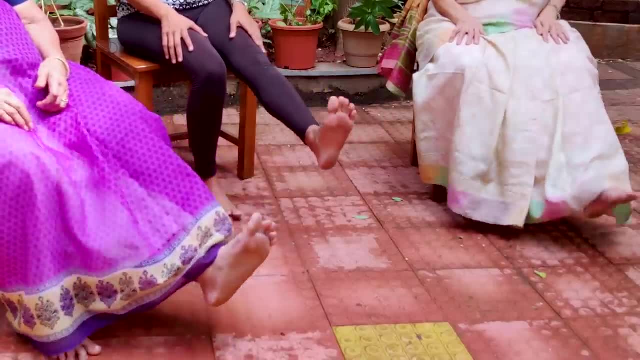 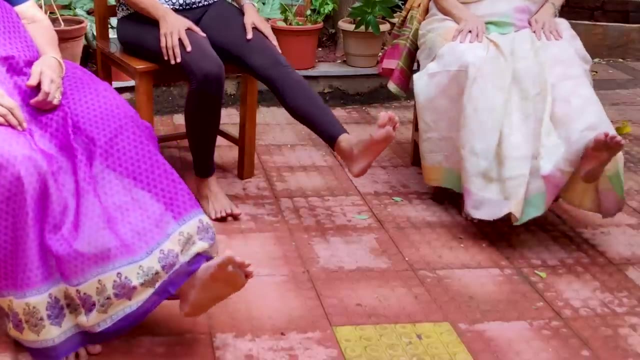 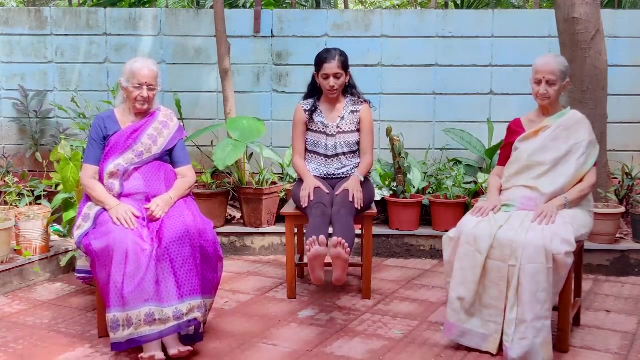 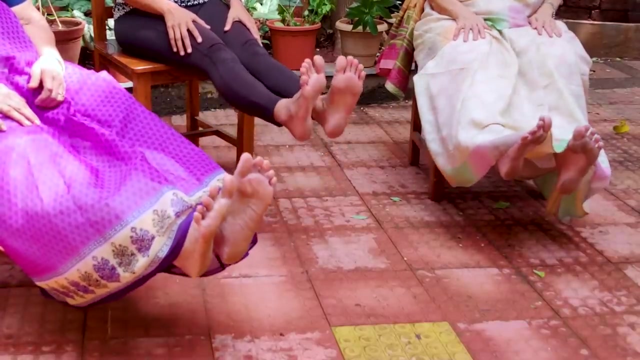 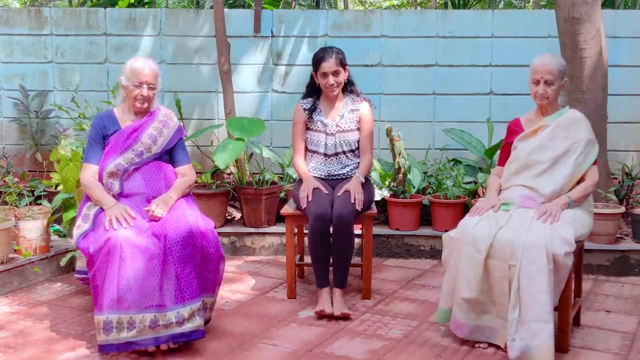 and relax other leg, left leg, up. flex your foot small circles and reverse and relax. raise both your legs up and get your legs down. keep going, raise both your legs up and down, up and down. we'll do seven more up and down and six and down and five down, four and down and 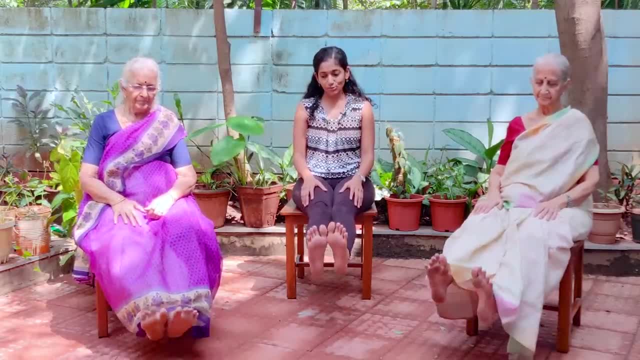 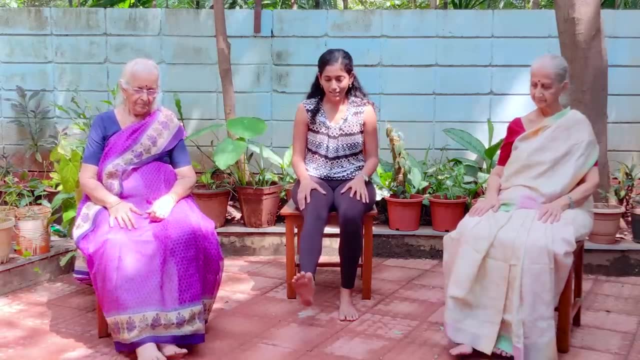 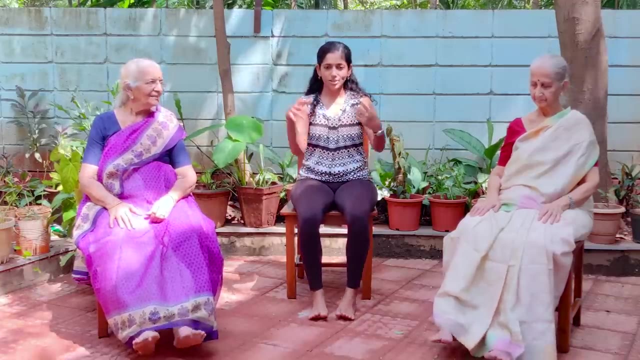 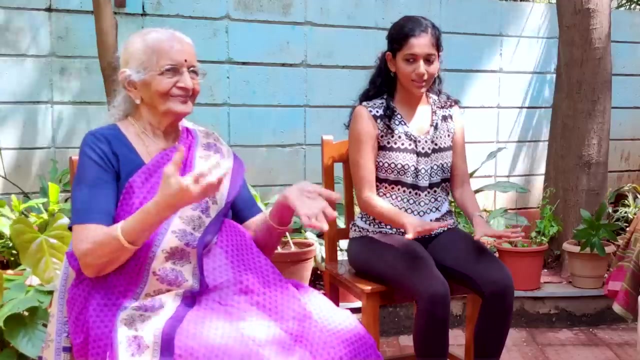 three down, two and down, last one and down, relax. shake your right leg out, shake, shake, shake. shake your left leg out. give your legs a good shake, very good, and shake your hands out. okay, and relax. we're going to do a few exercises for your face now we finish. 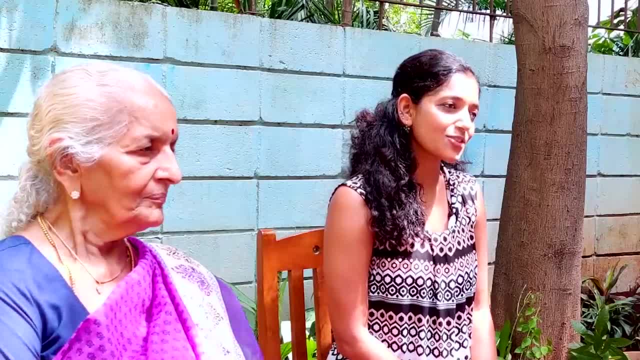 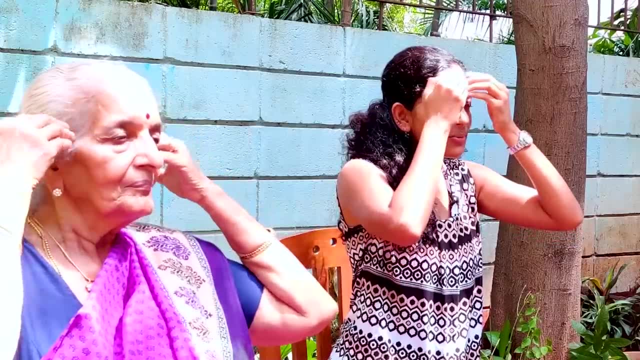 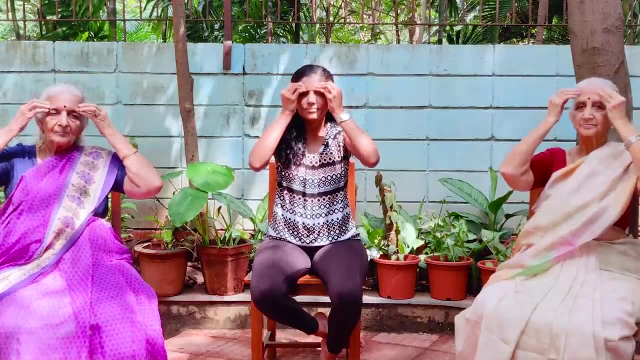 working on your hands and your legs. we'll do some relaxing exercises for your face, followed by a very simple pranayama. so four fingers at the center of your forehead start massaging your forehead, going from the center down to the sides. from the center, the sides keep going. 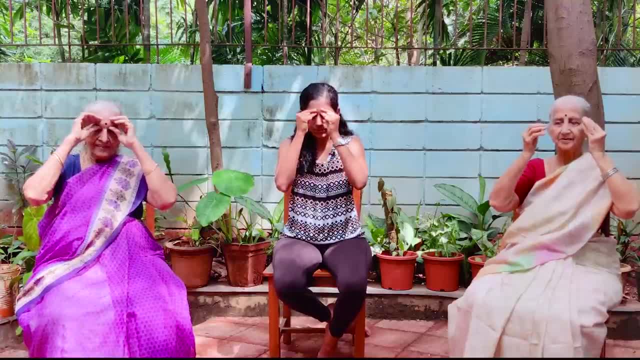 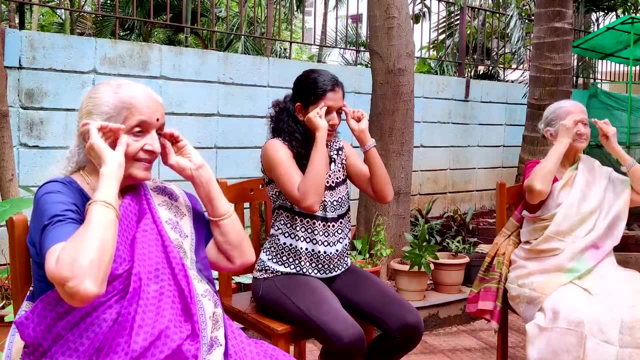 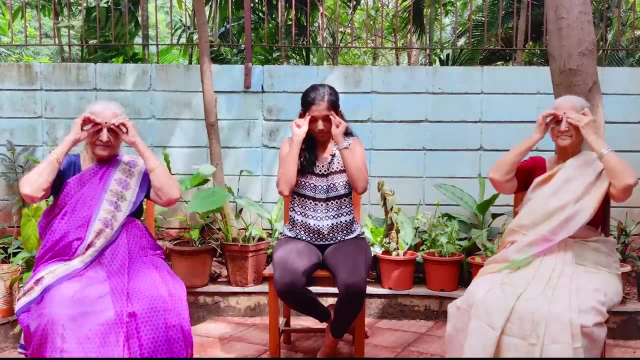 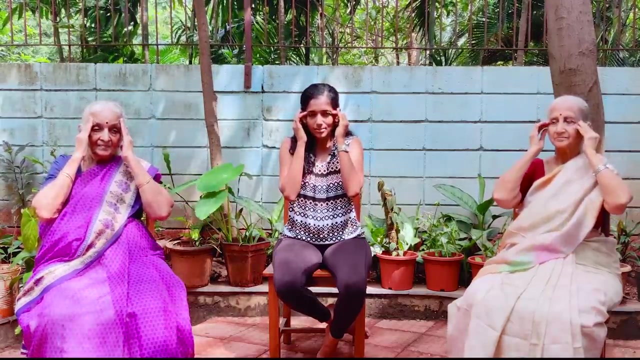 now use your index finger and your thumb, place it on your eyebrow and start running your fingers from the center again to the side, from the center down to the side, from the center to the side, taking your four fingers on the side of your forehead massage in a circular. 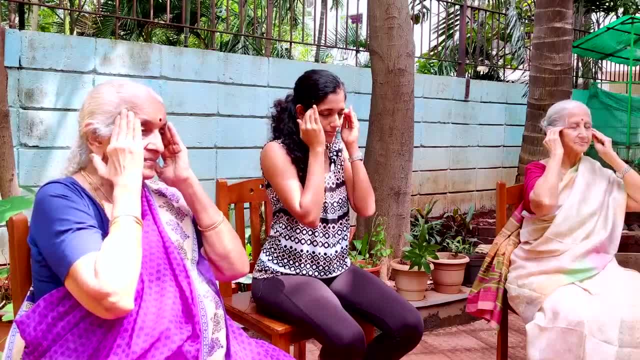 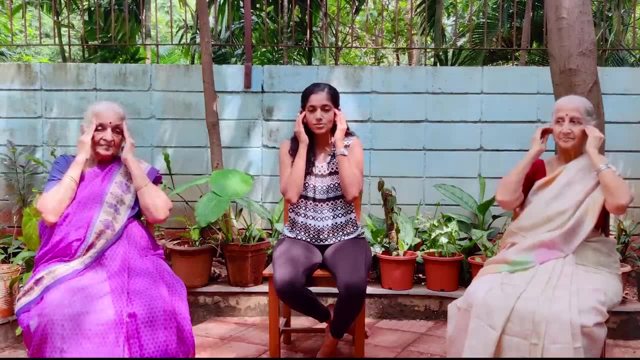 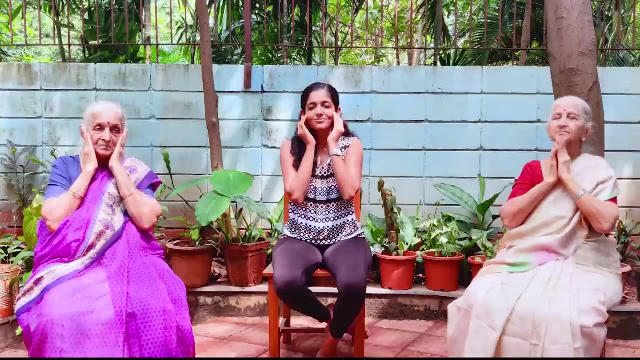 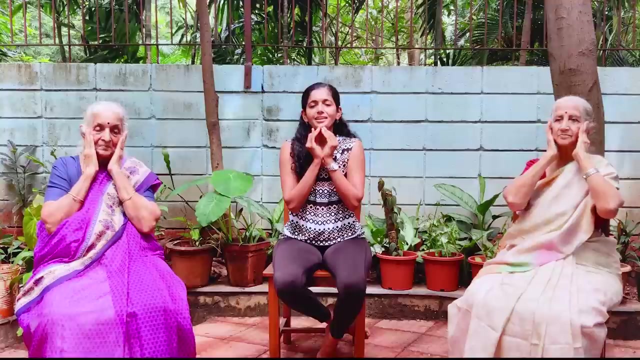 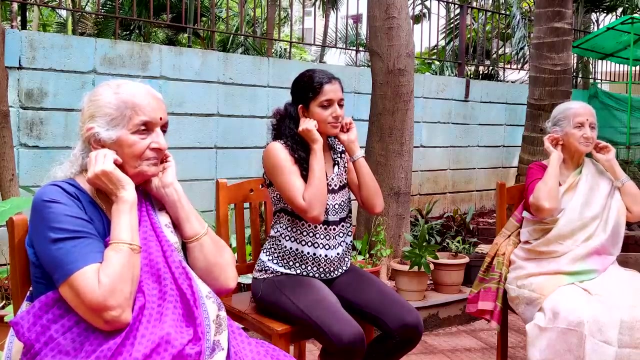 motion and relax your cheekbones, going from your cheek to your chin, again going down from your cheek to your chin. relax, grab hold of your ears and pull your ears down and relax. okay, we'll do a simple pranayama, we'll do alternate nostril breathing. so you take two. 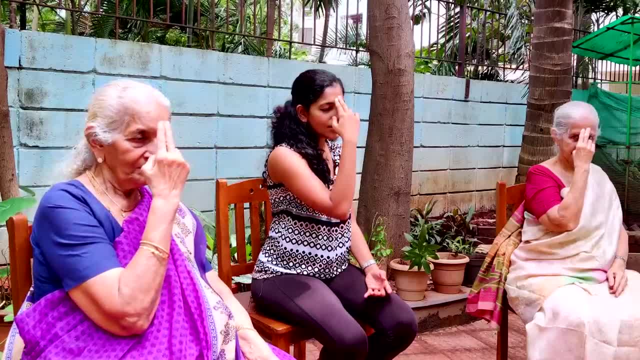 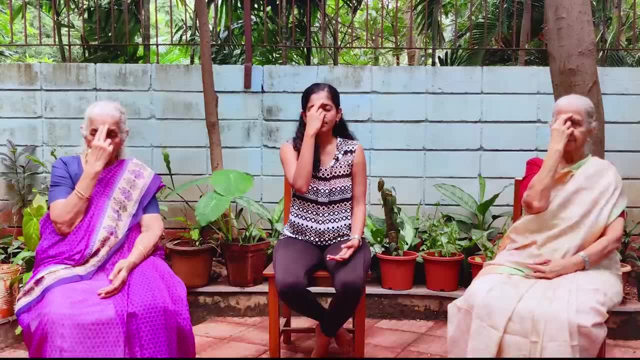 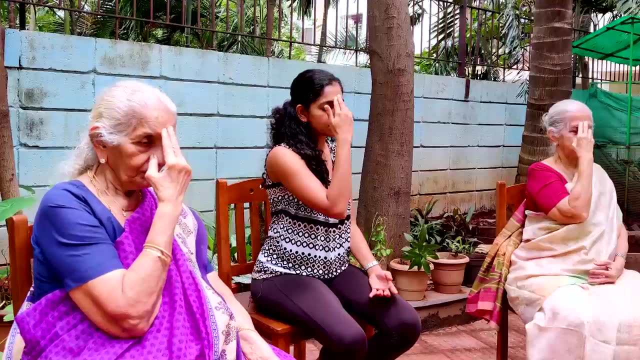 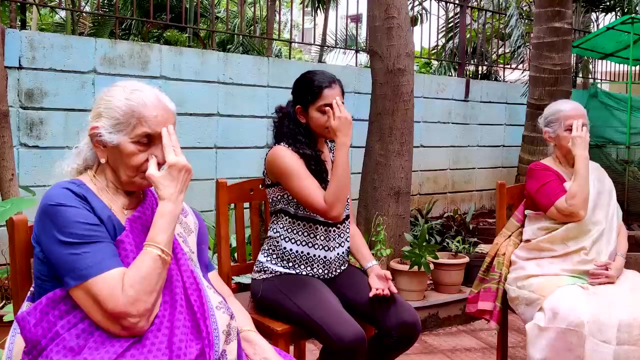 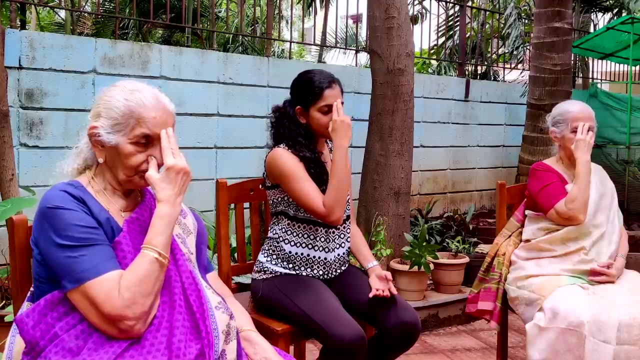 fingers at the center of your forehead, place your thumb on your right nostril, your other two fingers, closing your left. So first, inhale through your left, close left. exhale through your right. inhale right, close right, exhale left. That's one round, we'll. 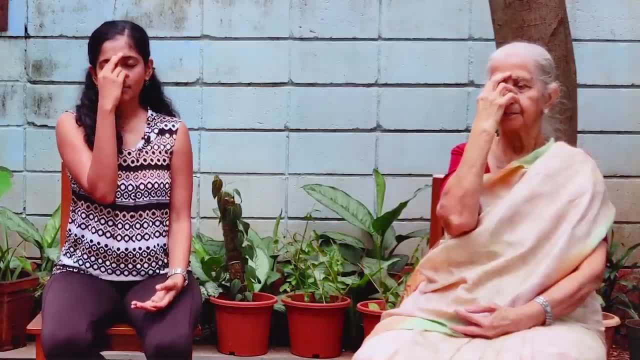 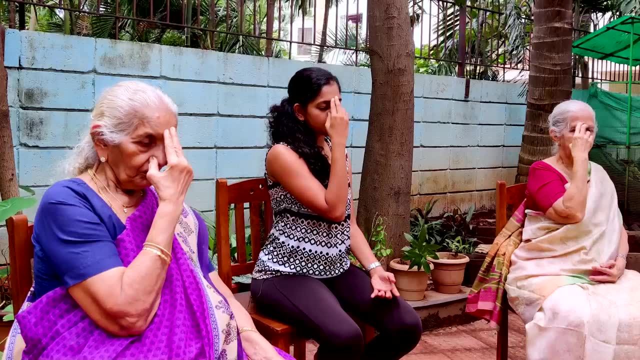 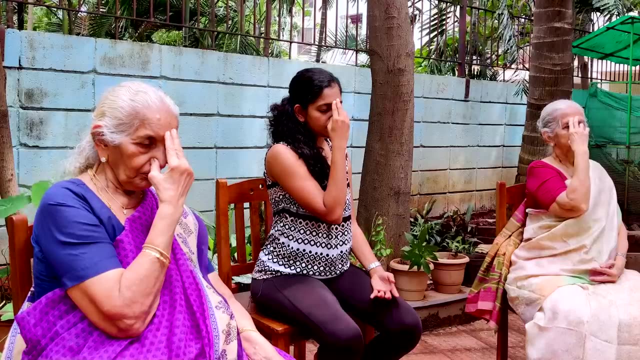 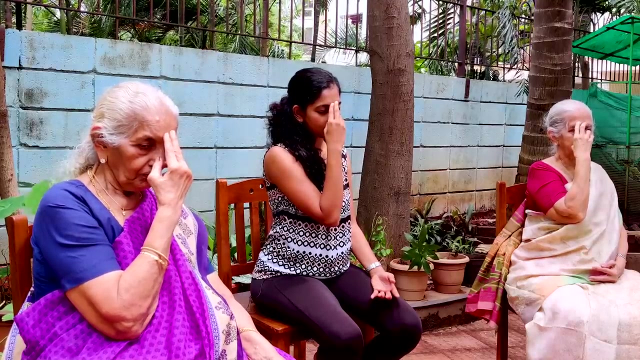 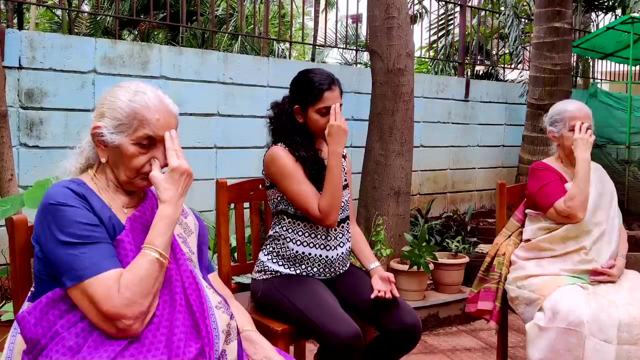 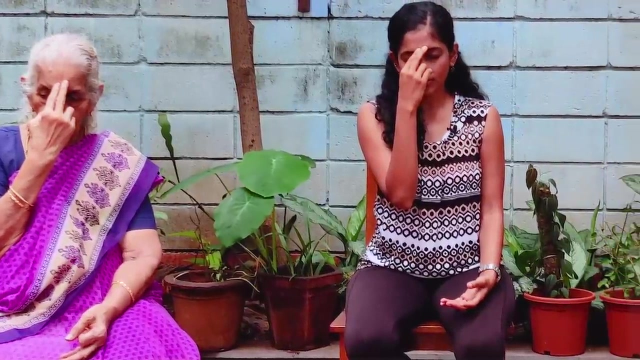 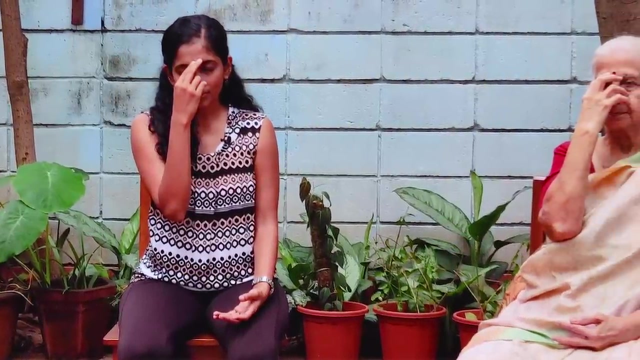 keep going with our eyes closed. Inhale left, close left. exhale right, close left. exhale right. inhale right, close right. exhale left. Inhale left, close left. exhale right, close left. exhale right. inhale left, close left. exhale right. inhale right, close left exhale. 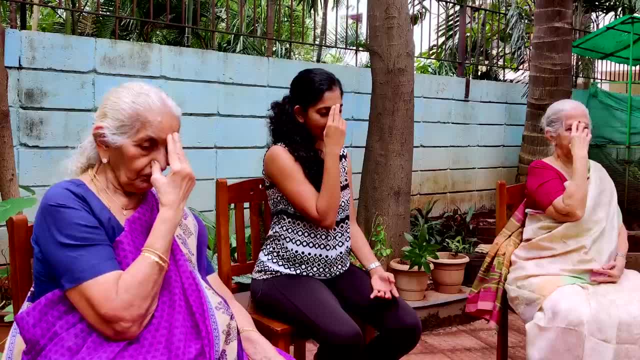 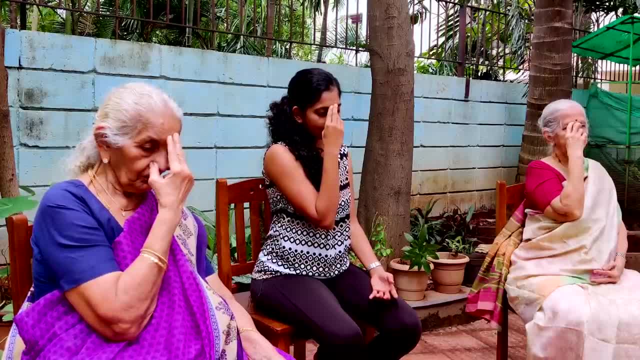 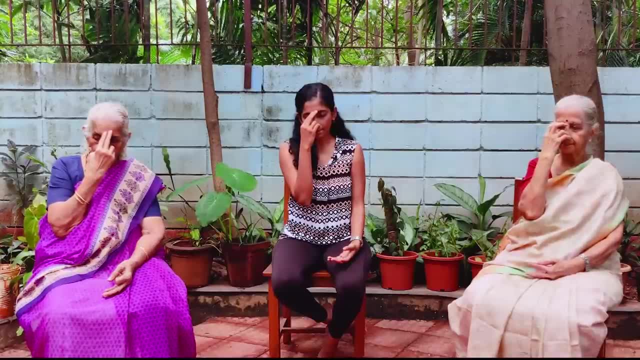 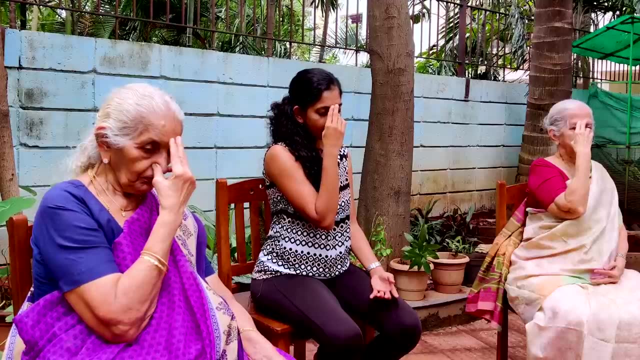 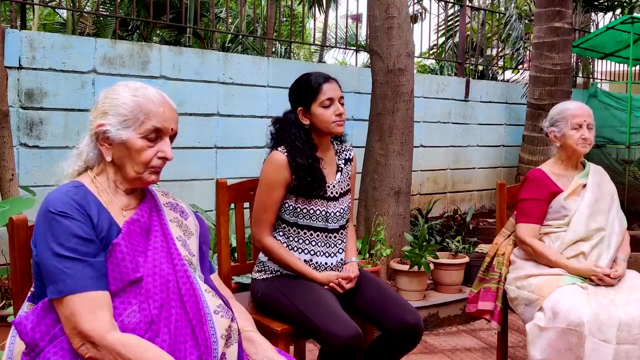 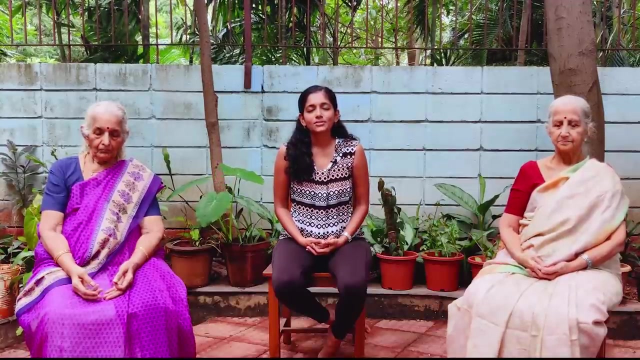 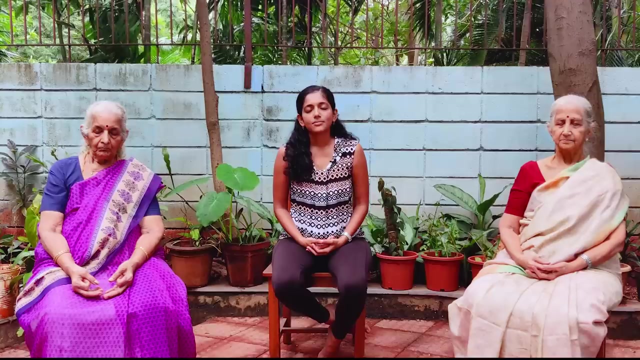 Inhale left- close left, exhale right. Inhale right- close right, exhale left. You can slowly keep your eyes closed, drop your hand down. Let's take a long, deep breath in and slowly breathe out. One more time: take a deep breath in and slowly breathe out.